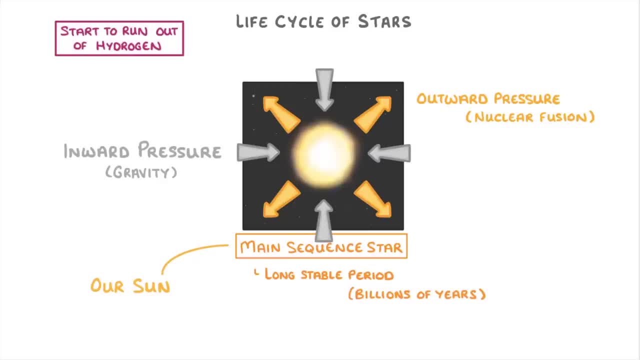 remember, is effectively its fuel. You don't need to worry about the details, but basically this means that the star won't be able to do any more nuclear fusion. This means that the star is likely to start to fuse around some preference of the points of the planet and whether or not it can be extinguished. 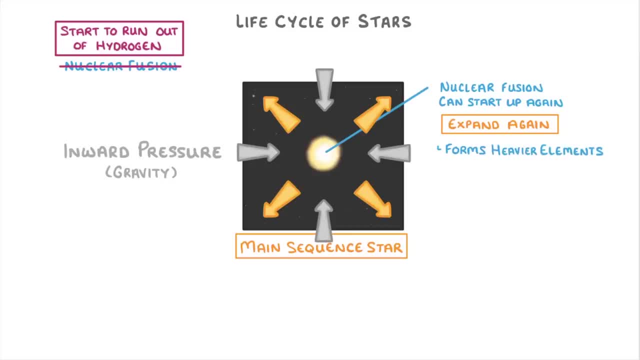 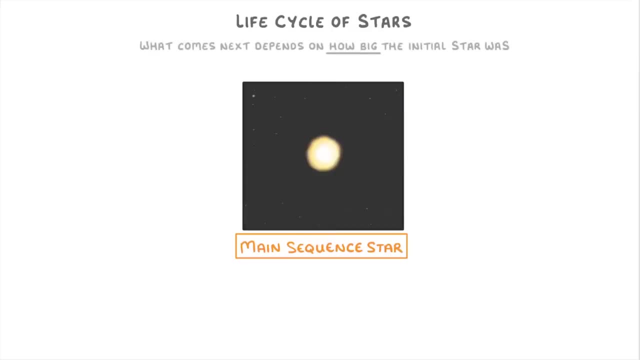 And so the inwards pressure of gravity takes over and contracts the star into a small ball until it's so hot and dense that the fusion can start up again, which will cause it to expand again. much the star expands depends on how big the initial star was. If it was a small to 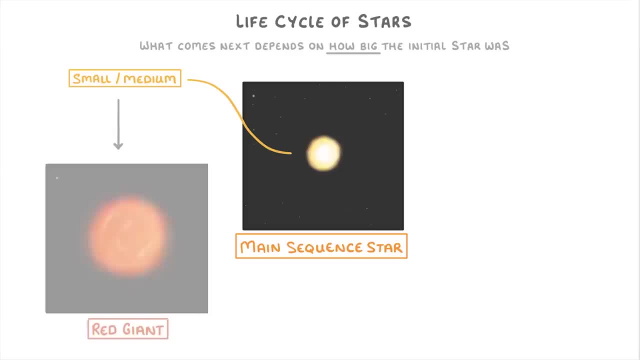 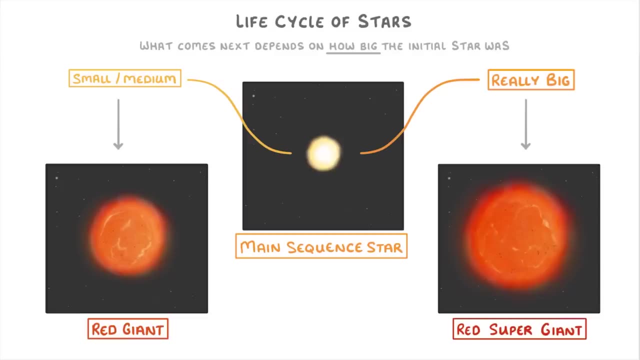 medium star like our Sun, then it will form a red giant. But if it was a really big star, then it would form a red supergiant. Each of these two types complete the rest of their life cycles in different ways, So we're going to take a look at the red giant first, and 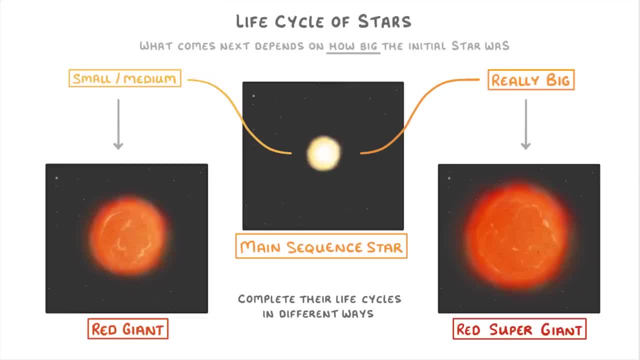 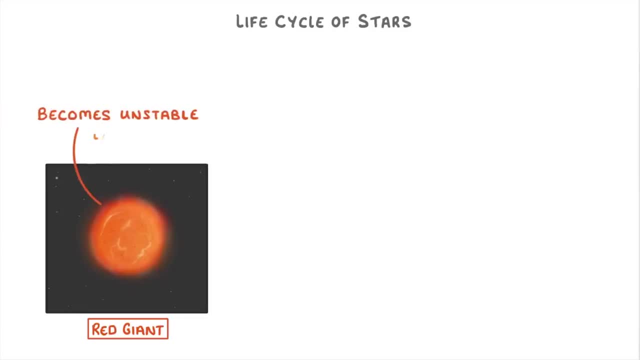 then we'll come back to the red supergiant. After a relatively short time, the red giant becomes unstable and expels its outer layers of dust and gas. This leaves behind a hot, dense, solid core which doesn't do any. 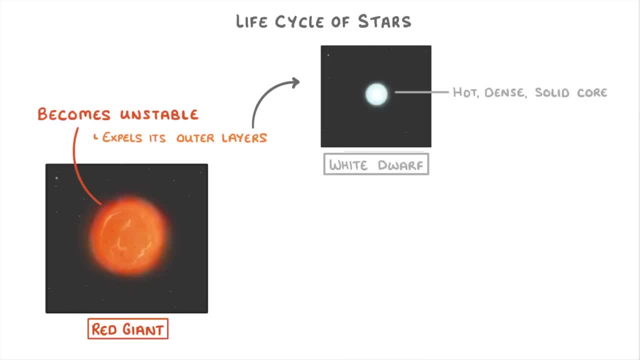 nuclear fusion. We call this a white dwarf because it gives off lots of light, so appears white and is relatively small. Over time the white dwarf gets cooler and darker as it emits all of its energy, until finally it transitions to a black dwarf because it no longer has enough energy to emit light. 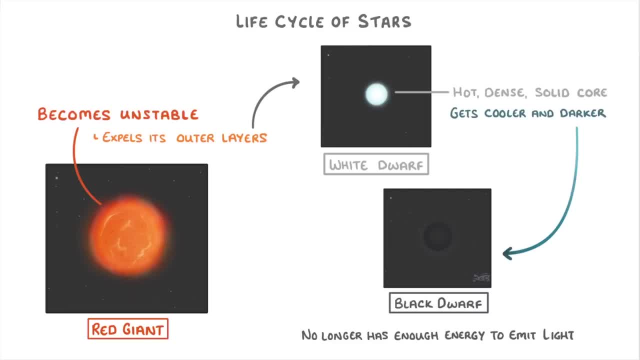 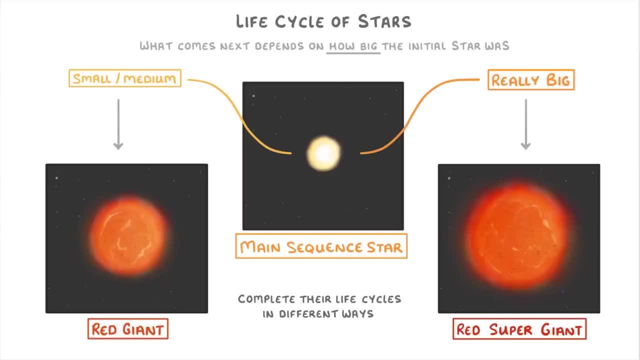 and so appears dark Now if we whiz back through the two options for our main sequence star, the other possibility for the really big stars was to turn into a red supergiant. So if we look at the red dwarf, we can see that the white dwarf has a lot of energy. 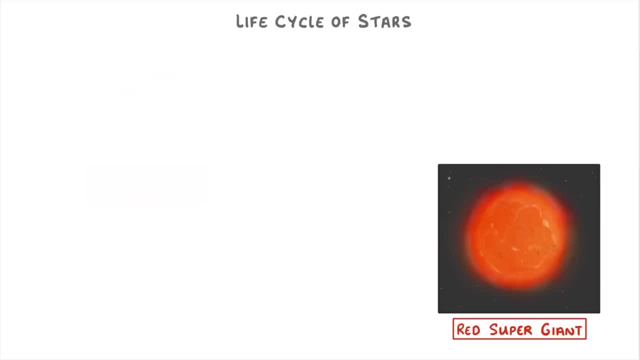 and is a little bit more powerful than the other two. So let's now look at these Red supergiants actually start to shine brightly again as they undergo even more nuclear fusion. After passing through several cycles of expansion and contraction, though, they eventually explode.